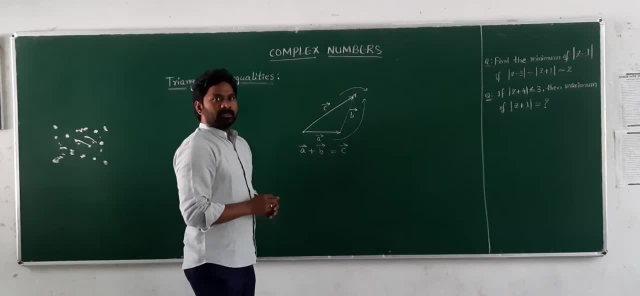 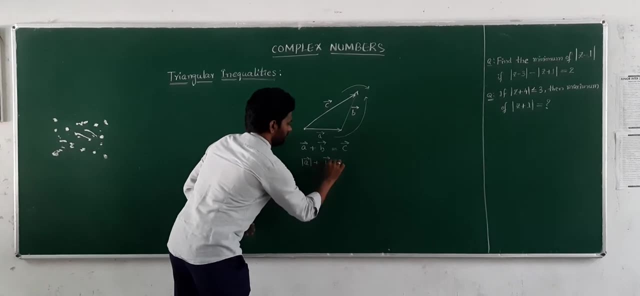 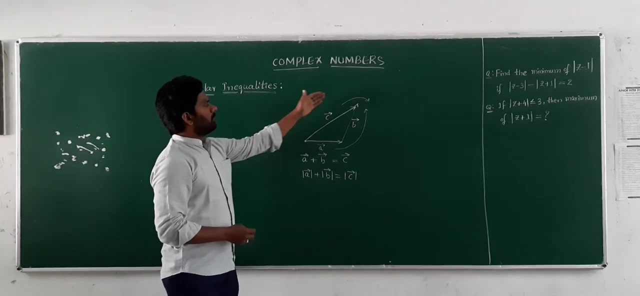 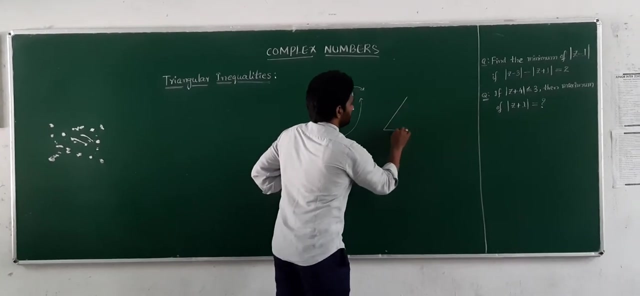 equals to vector c. So if I consider the magnitudes, then I can write this as: magnitude of vector a plus magnitude of vector b equals to magnitude of vector c. So this is from the law of addition, of law of triangles. So now, if we consider the triangle, if we 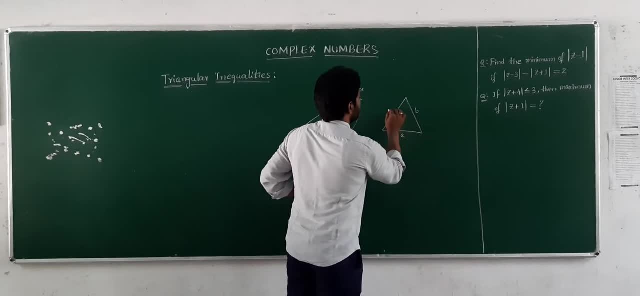 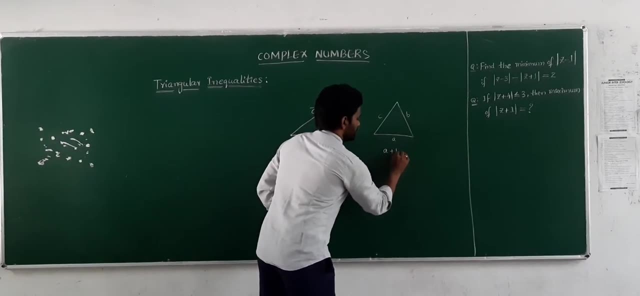 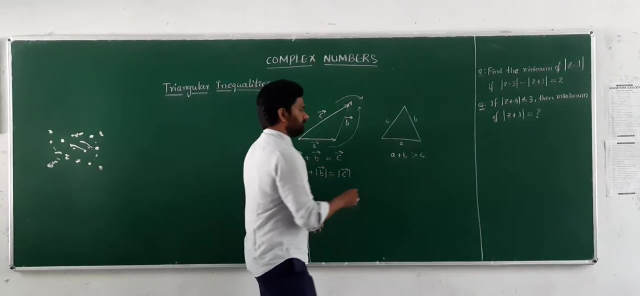 consider the triangle of sides a, b, c, of sides a- b c, and we know that the sum of any two sides- So this must be greater than the another side, third side, and the difference between the any two sides is always less than the another side. So you have to consider some. 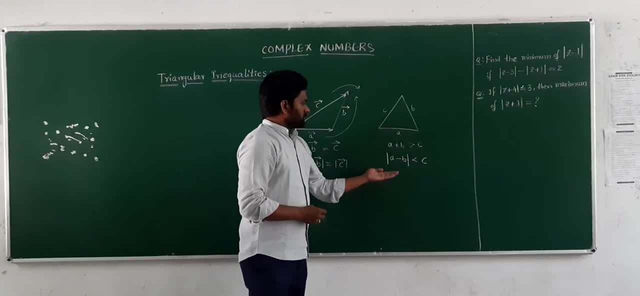 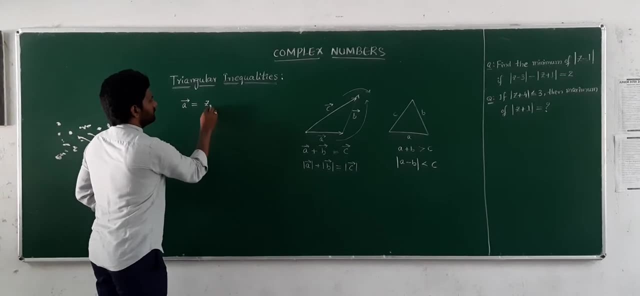 magnitudes. So now applying these concepts, now I am considering: so vector a as a complex number- z1, okay. and vector b as a complex number- z2, okay. So vector b as a complex number- z1, okay. So vector b as a complex number- z2, okay. So vector b as a complex 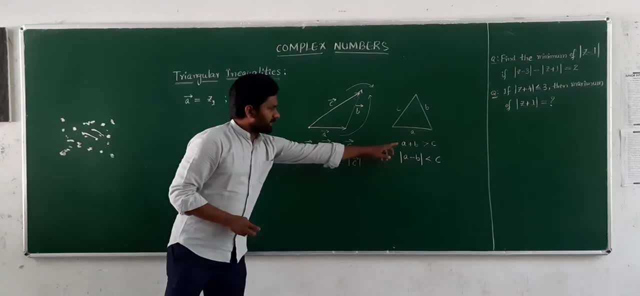 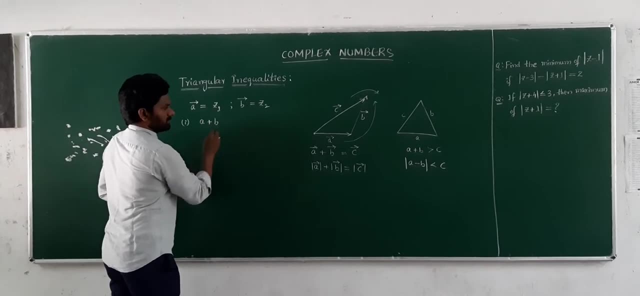 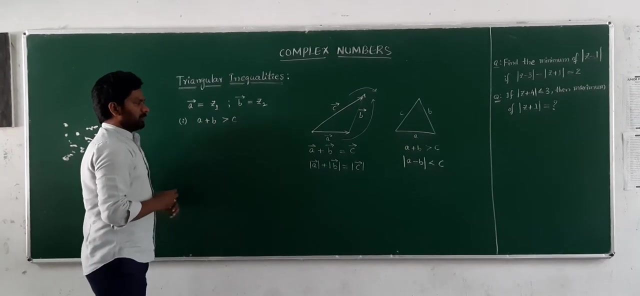 number z2,. okay, So now I am considering the case 1, where it is the first one, the sum of any two sides is greater than the other side. sum of any two sides is greater than the other side. So from this one, if we apply to the law of addition of vectors, so regular. 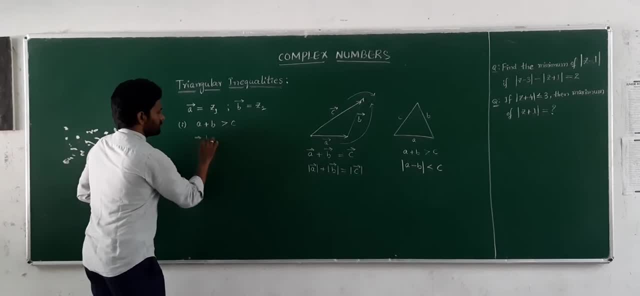 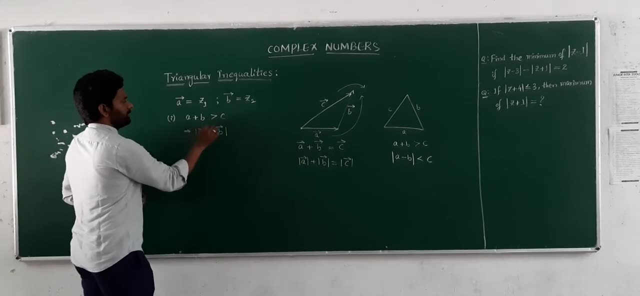 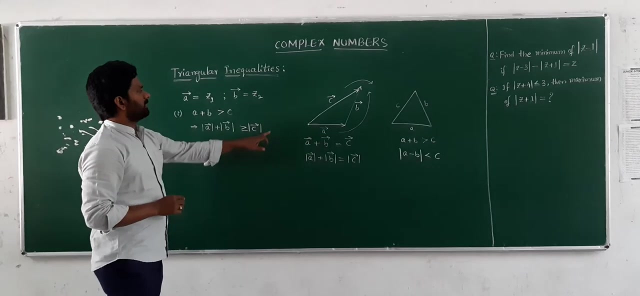 law of addition of vectors, then I can write this as so: vector a plus vector b, magnitude. so just, I am considering the magnitudes which greater than or equals to the vector c. Okay, now I am replacing, applying this to the complex numbers. Now a is replaced by vector, a is 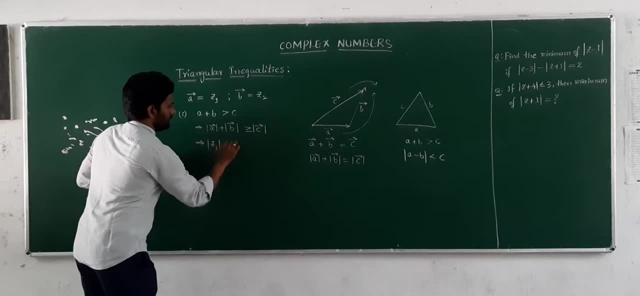 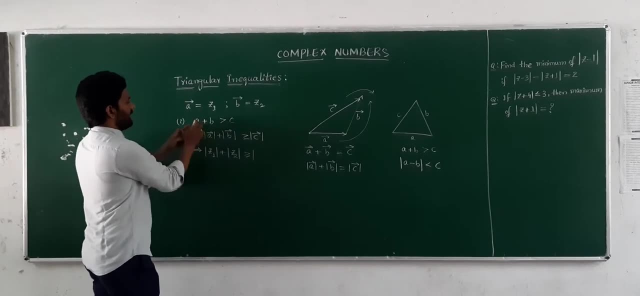 replaced by complex number z1 and vector b is replaced by complex number z2, which is greater than or equals to, where c is nothing but a plus b, c is nothing but a plus b, a is nothing but z1 plus b is nothing but z2.. 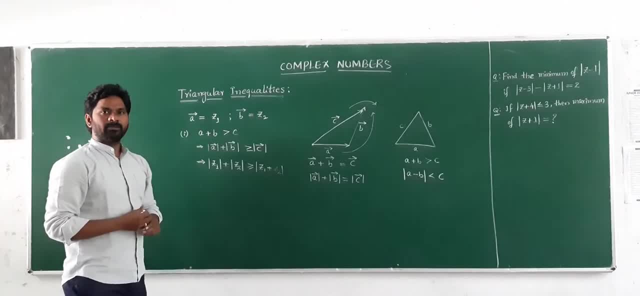 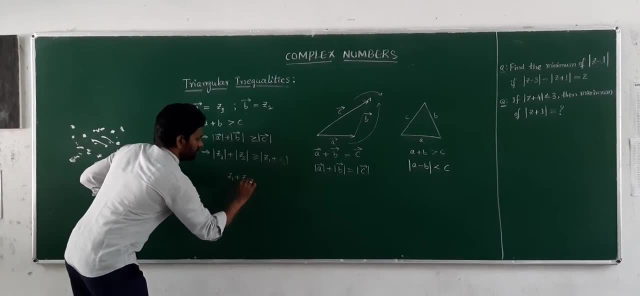 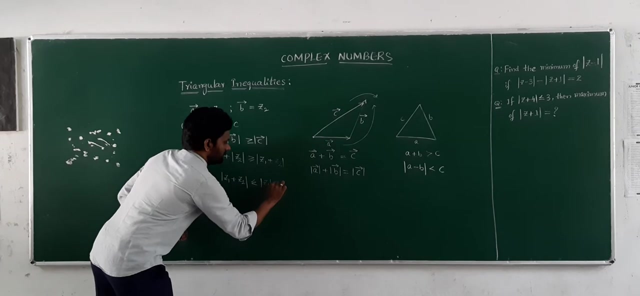 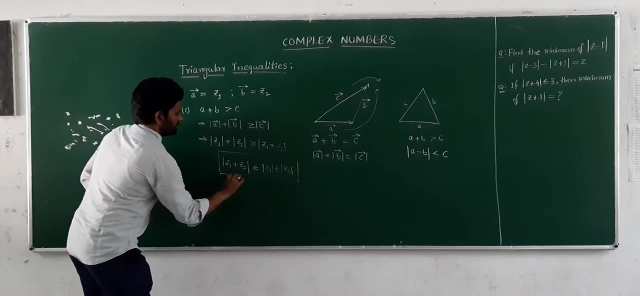 Okay, a is nothing but z1 and b is nothing but z2.. And we can come to that from this one, the modulus of z1 plus z2 is less than or equals to, modulus of z1 plus modulus of z2.. So, which is one of the triangular inequalities? Okay, so, like I have said this, 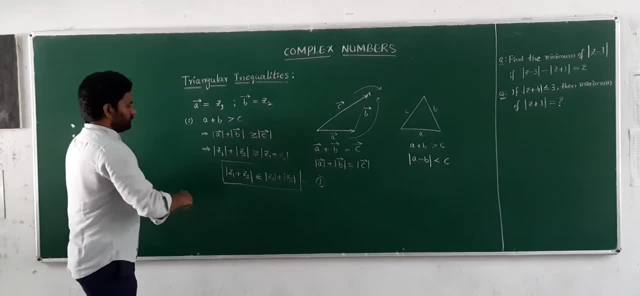 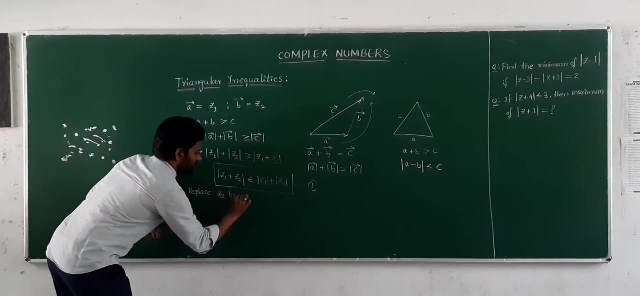 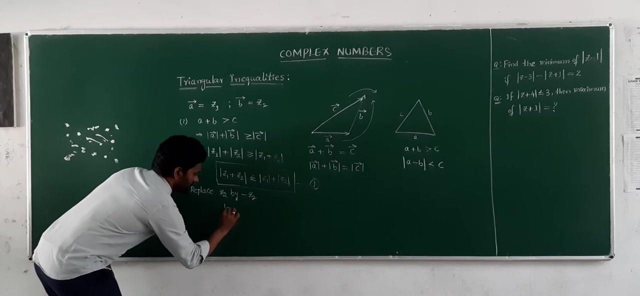 is first, triangular inequality. So if I replace, if I replace z2 by minus z2, okay, if I replace the z2 by minus z2, then what I will get over here: z1 plus z2 is replaced by minus z2, z1 minus z2, difference. 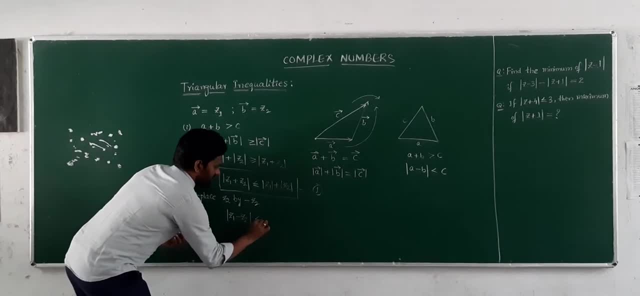 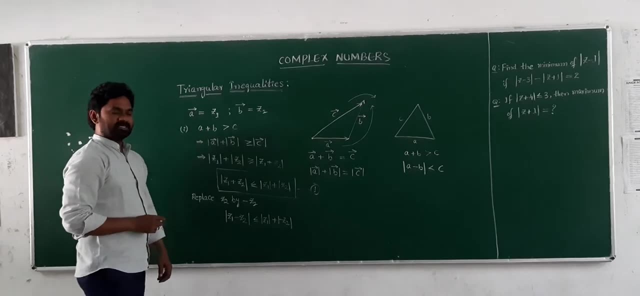 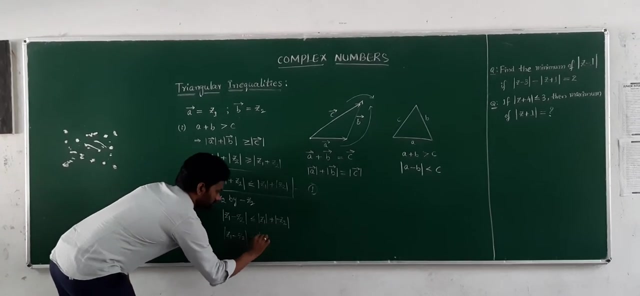 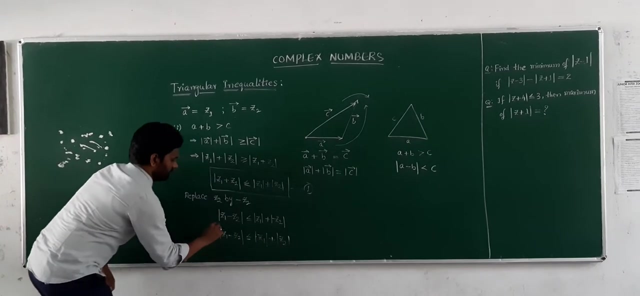 between the complex numbers, modulus is less than or equals to modulus of z1 plus mod of minus z2.. So which is also written as z1 minus z2, less than or equals to mod of z1 plus mod less of a negative number or less is a consider as a plus itself. then we can write. we can. 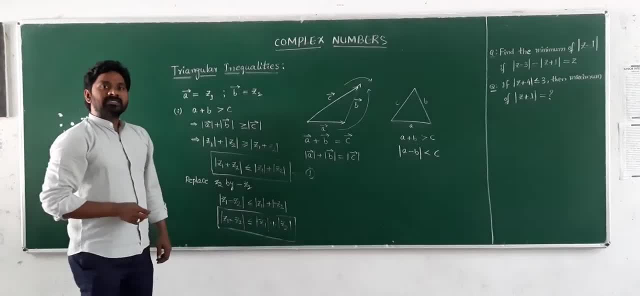 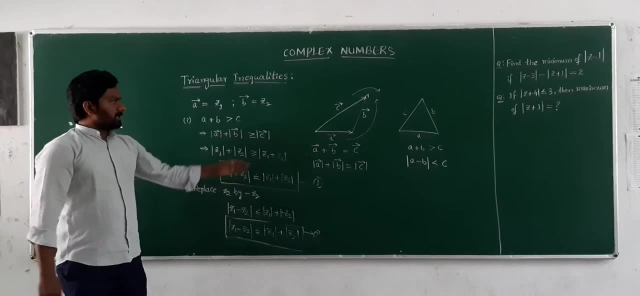 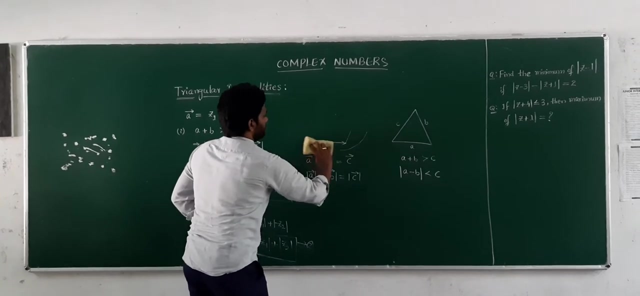 write mod of z1 minus z2, less than or equals to mod less of z1 plus mod less of z2, which is equals to. now we can consider it as a either regular inequality. Okay, So now, if I cancel out the case two, what is the difference between the any two sides? 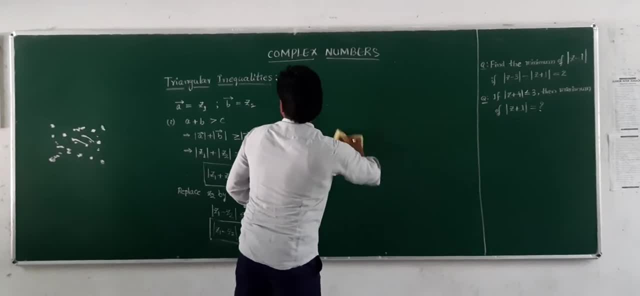 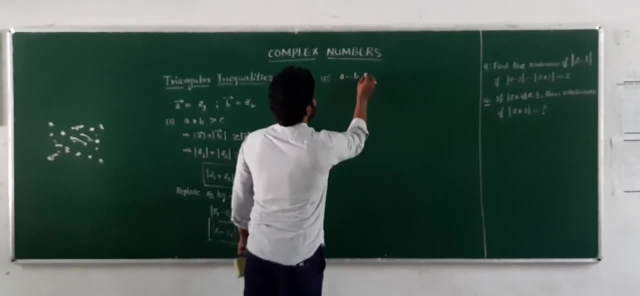 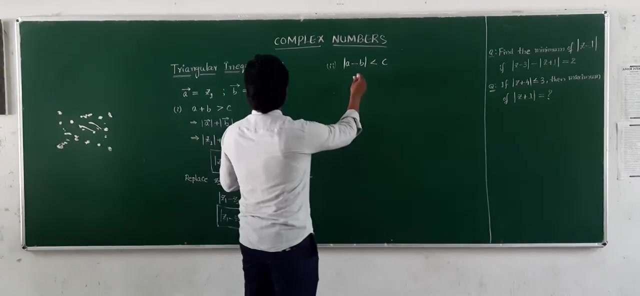 Difference between the any two sides is less than the third side. Now I am canceling from the triangle what it is. a minus b is less than c. Now I am making the magnitude difference. Okay, So now I am replacing with the vectors. I can write it as vector a: i's. 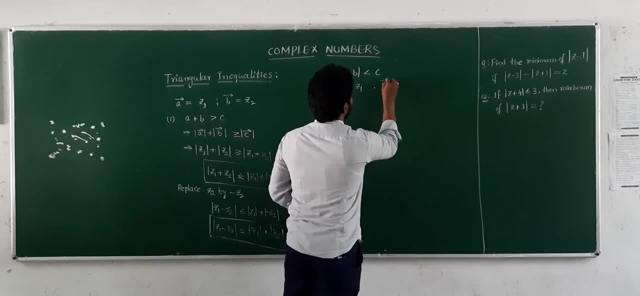 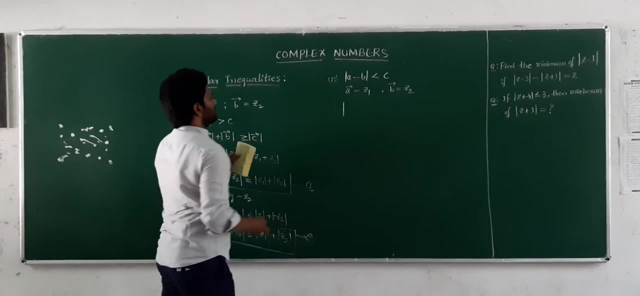 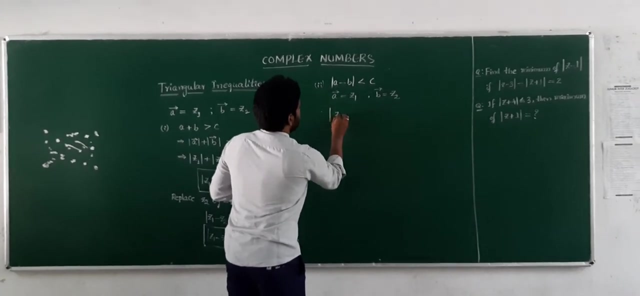 Complex number z1, and vector b i's complex number z2.. So now modulus of a is nothing but amplitude. So that means nothing, but a is the value. So to get the vector a value now we need to replace s What it is: a i's modulus of z1 and b i's modulus of z2. 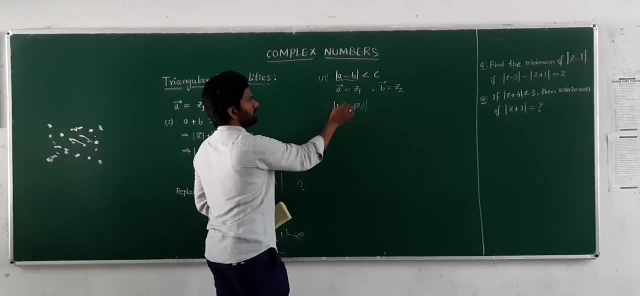 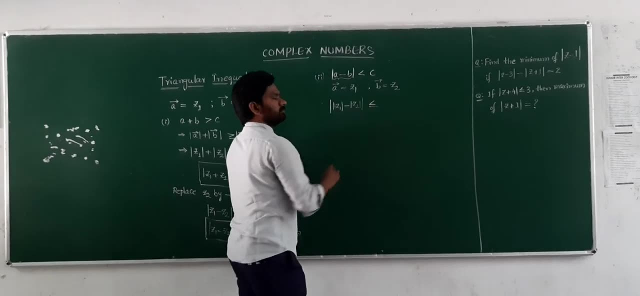 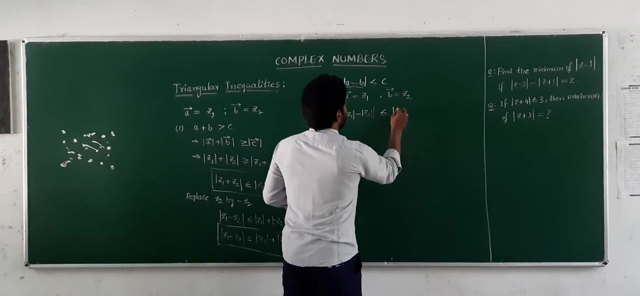 all modulus. So here a is replaced with modulus of z1, b is replaced with modulus of z2.. Right, All modulus is less than maybe or equals to c. What is c is the value. Then we can write it as: c is nothing but a plus b. So a plus b is nothing but z1 plus z2.. Okay, 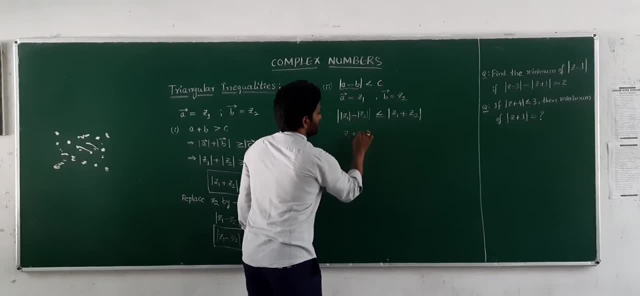 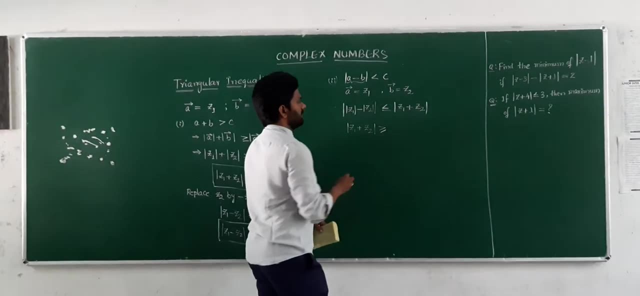 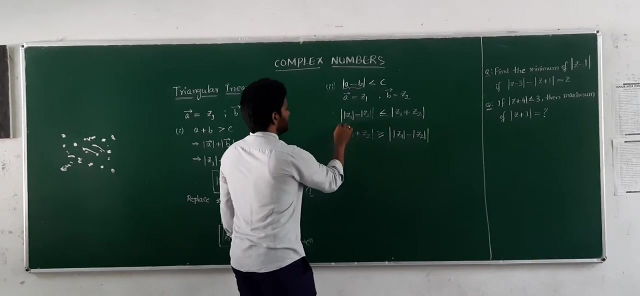 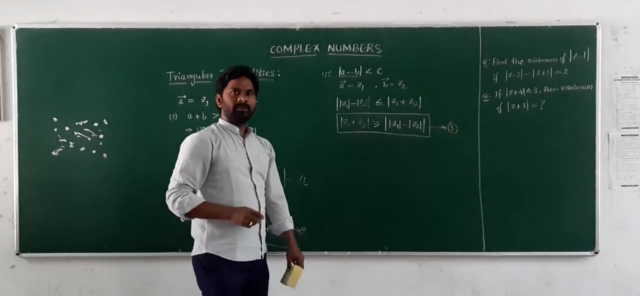 So if we rearrange this, we can write as: modulus of z1 plus z2 is greater than or equals to, Modulus of z1 plus z2 is greater than or equals to Modulus of mod z1 minus mod z2.. So, which is under and the inequality, And this will be less than 3.. Okay, And 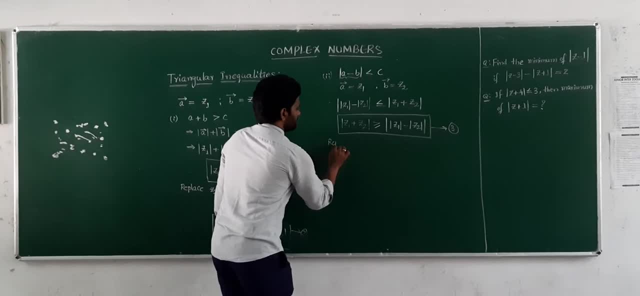 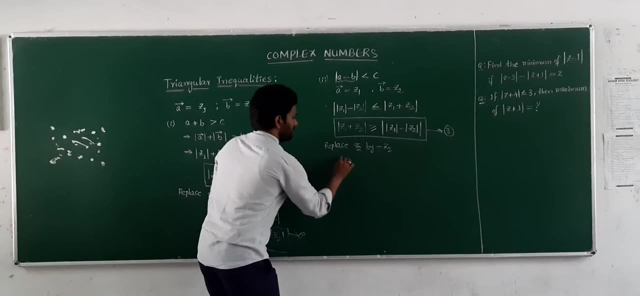 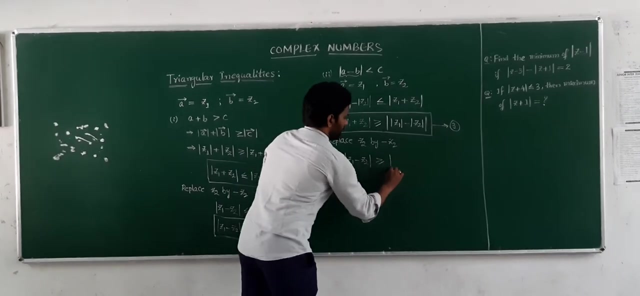 that will be less than 3.. So next, if we replace the z2 by minus z2.. Okay, Then what we get? I substitute in 3 z1.. z2 is replaced by minus z2. Then that is equal to modulus. 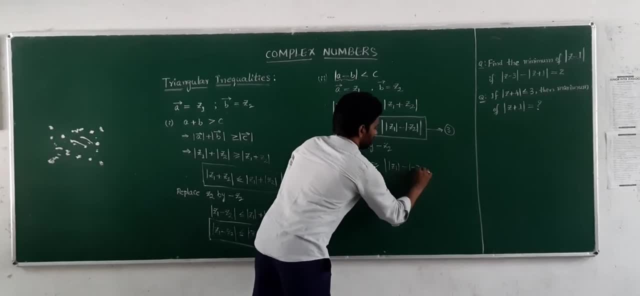 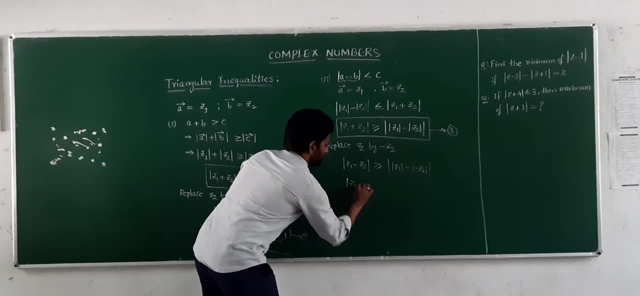 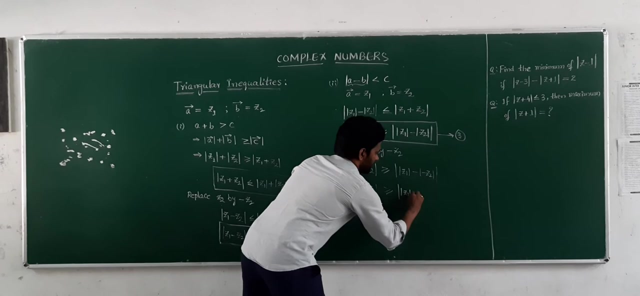 of mod z1 minus modulus of z2.. Okay, Modulus of mod z1 minus modulus of z2,, which is equals to z1 minus z2, is greater than or equals to modulus of mod z1 minus modulus of z2.. So, 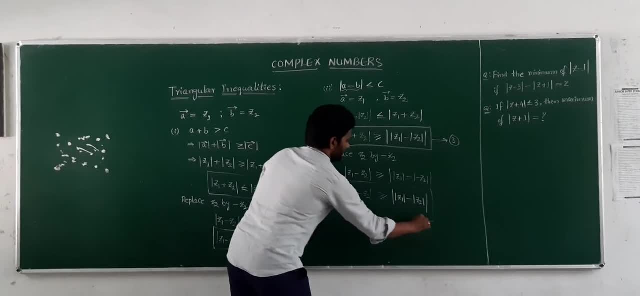 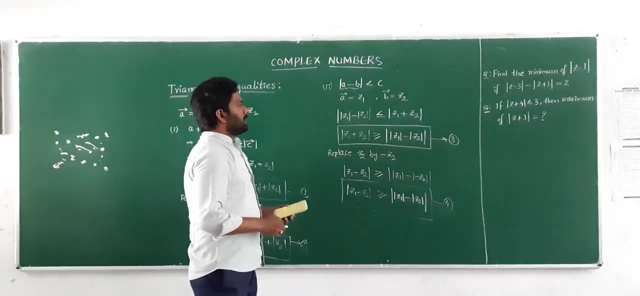 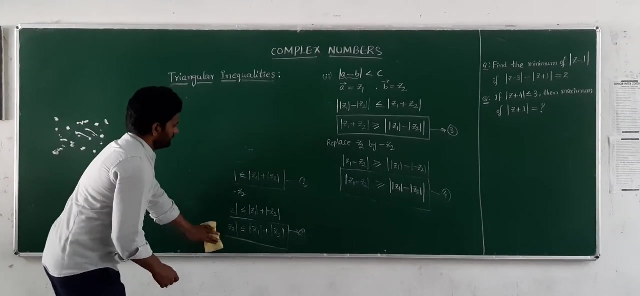 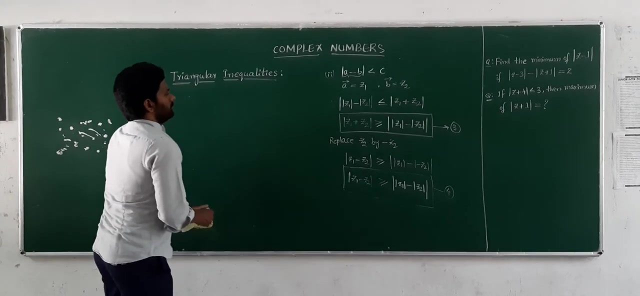 we can write this is as another triangular inequality. So now we are having fourth triangular Inequalities. Okay, Let I will summarize all these triangular inequalities, So in a better way to understand. So first consider, Okay, First consider z1, modulus of z1 and 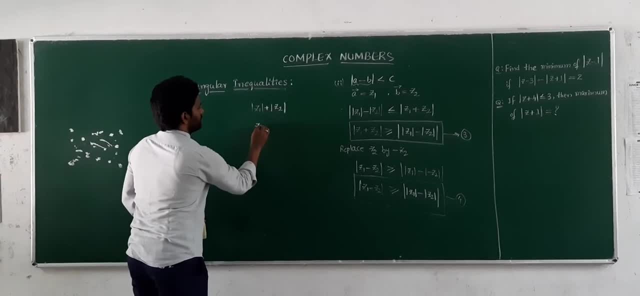 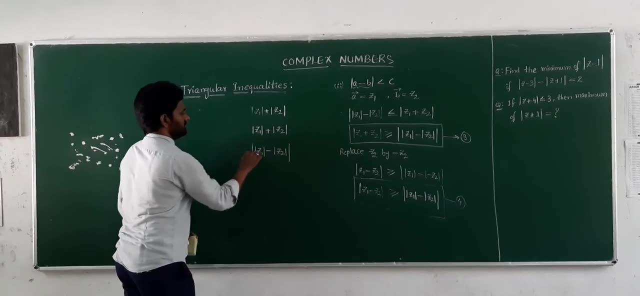 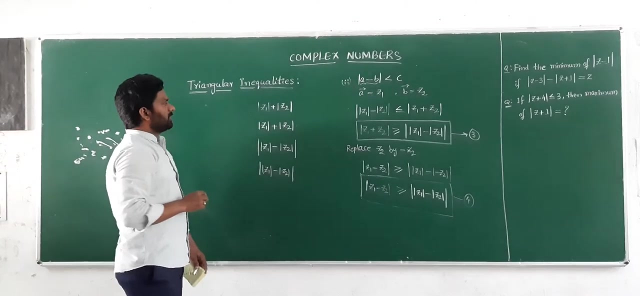 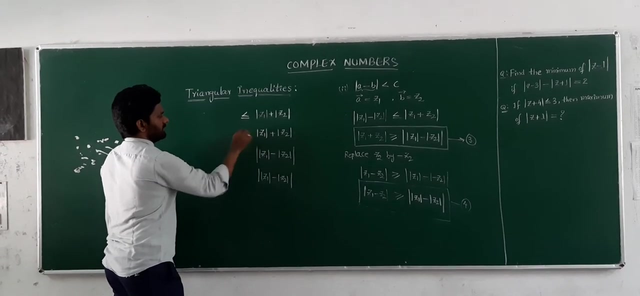 modulus of z. Write it again So: modulus of z1 plus modulus of z1 minus modulus of z2, whole modulus, And modulus of z1 minus modulus of z2, whole modulus. Okay, So whenever here we are having plus, then take s less than or equals to plus. Take it as less than. 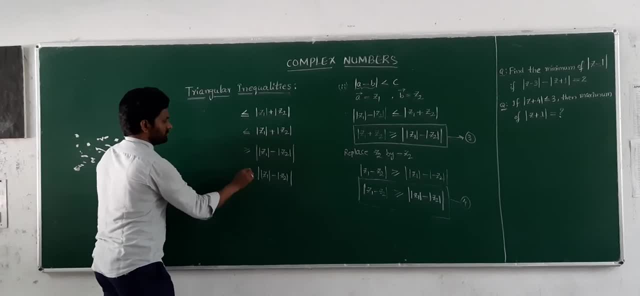 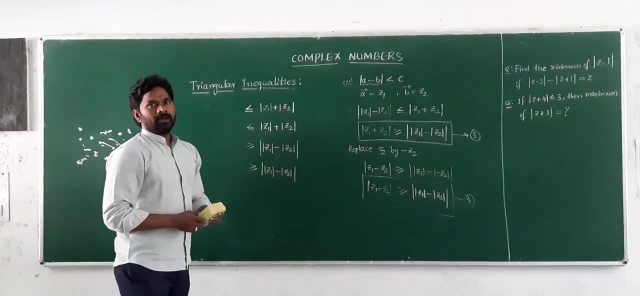 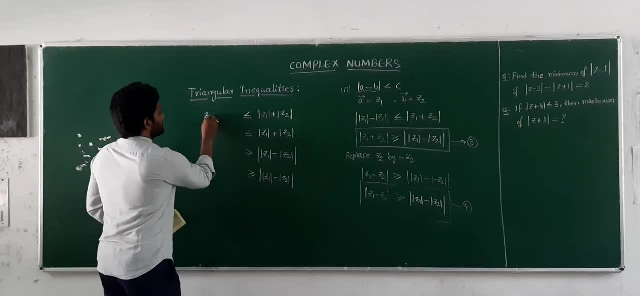 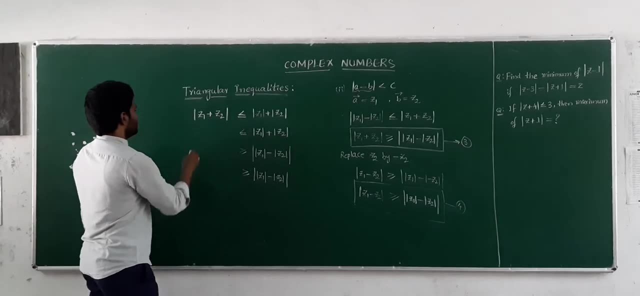 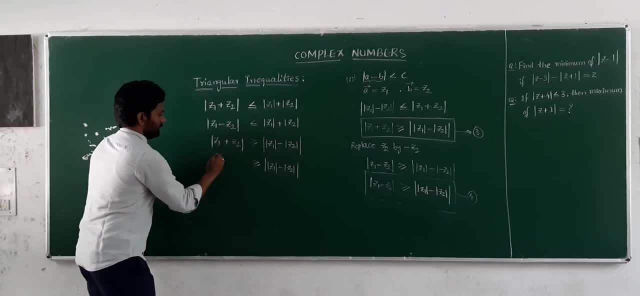 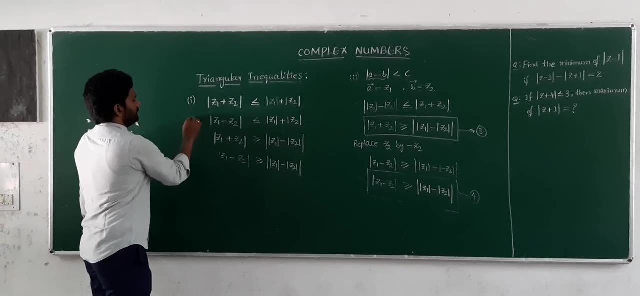 z2.. Okay, And z1 minus z. Okay, So you are having fourth triangular inequalities. So these are the z1 and z2.. Next we have the z3 plus z2.. Okay, So this will be z1. minus z2.. I have to cancel out z1.. So I have to cancel out z2.. Next I have to do z1 minus z1., So z1 minus z2.. Next I have to cancel out z1 minus z2. And z1 minus z2.. So. 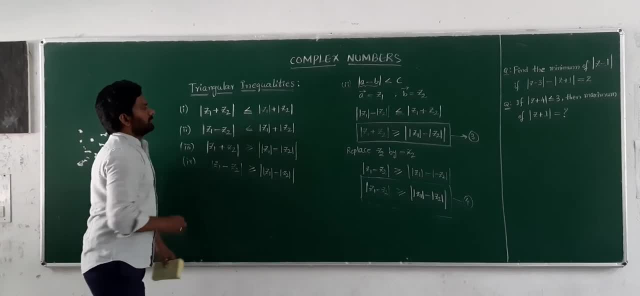 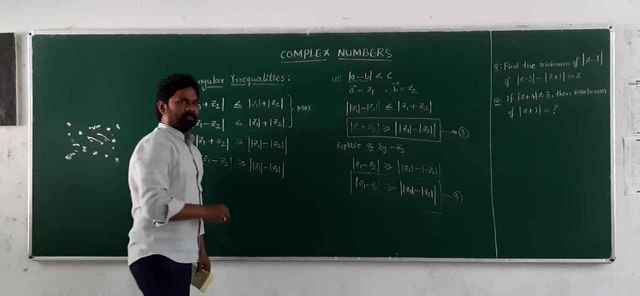 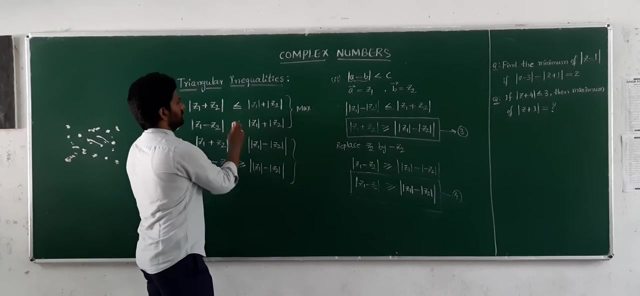 the four triangular inequalities. From these four, the first two: less than or equals to gives us the maximum values of the complex numbers. and less than or equals to gives us the sorry. less than or equals to gives us the maximum value. and greater than or equals. 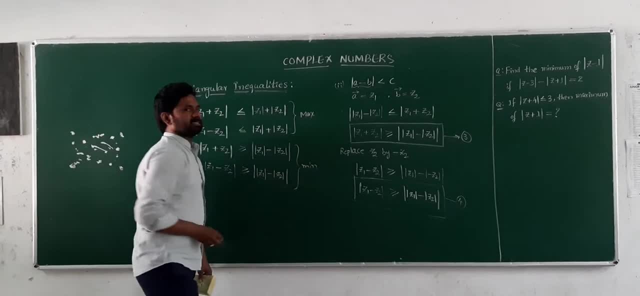 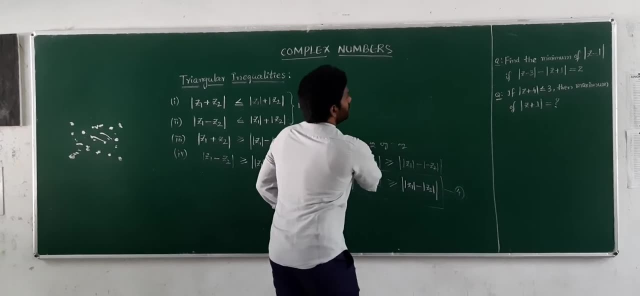 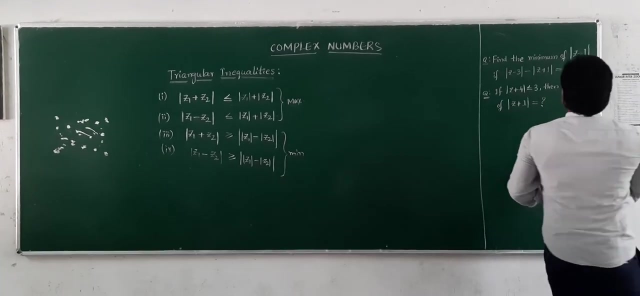 to gives us the minimum values of the complex numbers. Okay, So consider the question here. what is the question? Find the minimum of? here the question is, given that, find the minimum of mod of z minus 1, find the minimum of mod of z minus 1 if mod of z minus 3 minus. 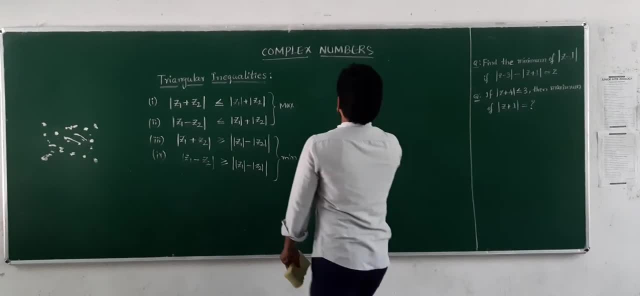 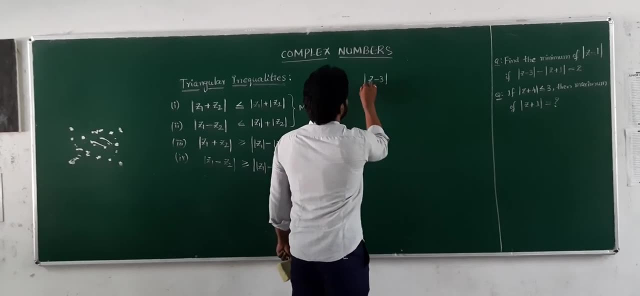 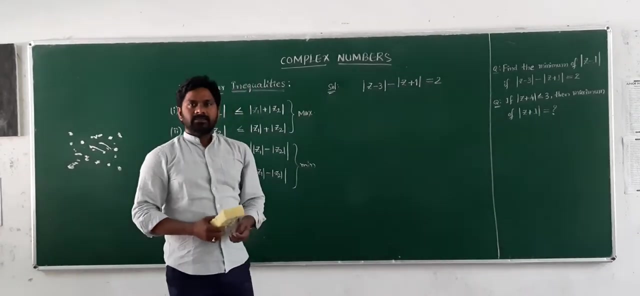 z plus 1 equals to 2.. In the question it is given that okay mod of that means modulus of z minus 3 minus modulus of z plus 1.. So if we consider this is as a complex number z1 and it is as a complex number z2, we can. 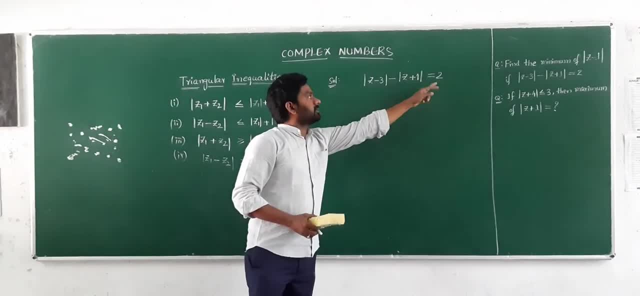 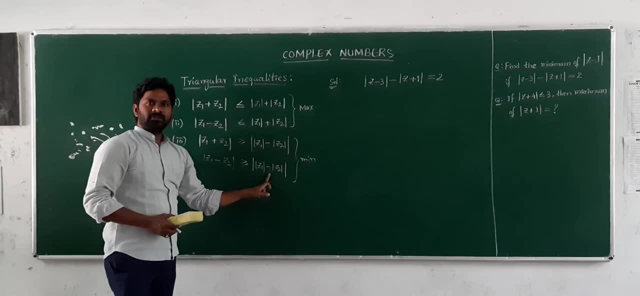 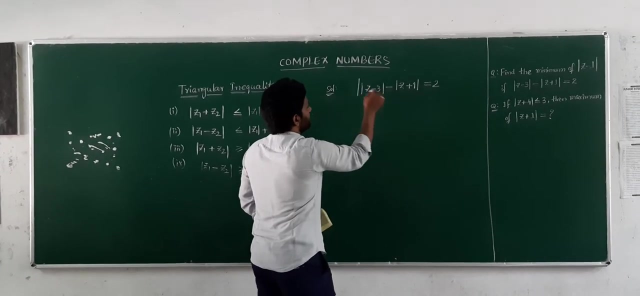 write as mod of z1 minus mod of z2 equals to 2.. So mod of z1 minus mod of z2, either it is the third inequality or the fourth inequality, either it is third and fourth inequality. So for a better understanding, I am considering this less. I am taking it as a modulus, nothing. 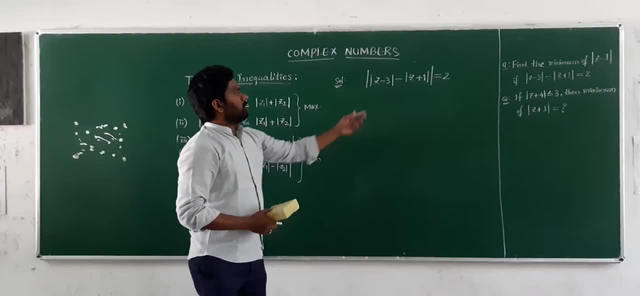 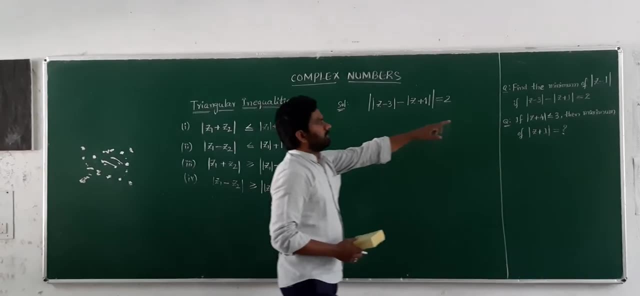 changes, the value will not change. Now it is in the form of mod of z1 minus mod of z2, either it is a third inequality or a fourth inequality, But our requirement: we need to obtain z minus 1.. So if I consider 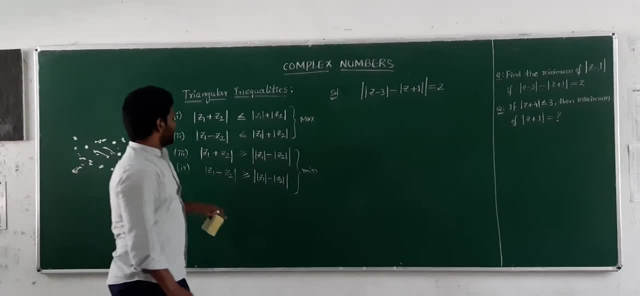 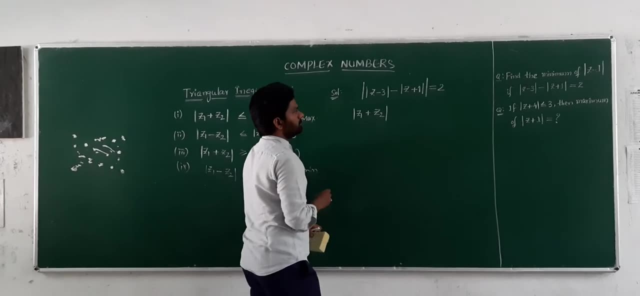 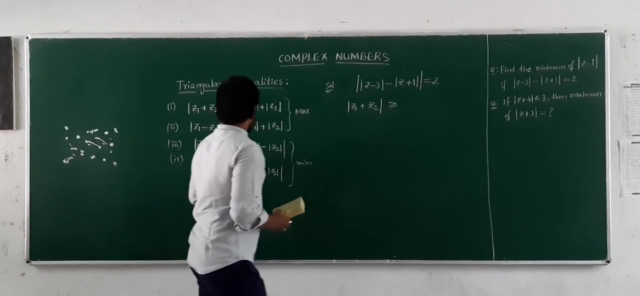 the third inequality: z minus 1,. if I consider the third inequality, what is the third inequality? z1 plus z2, mod of z1 plus z2 is greater than or equals to clearly that we need to obtain the minimum value. Minimum value means greater than or equal to z1 minus z2.. So 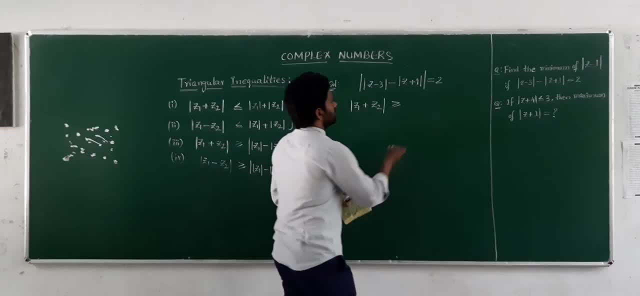 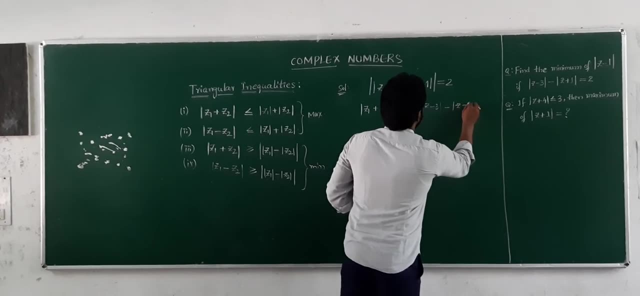 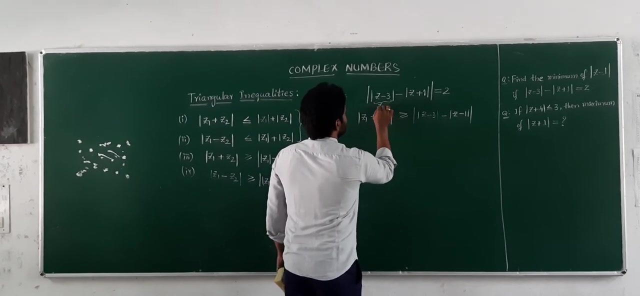 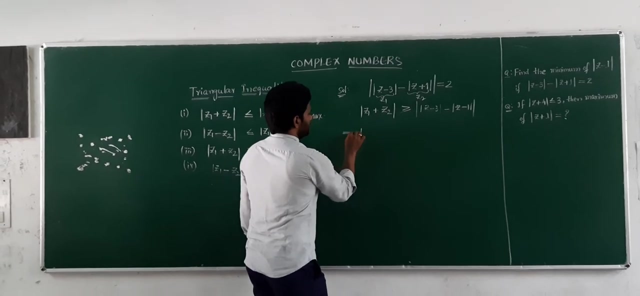 greater than or equal to, gives us the minimum value. So greater than or equals to mod of z1 minus 3 minus mod of z minus 1.. Okay, so this is it Clearly where I am considering this: z minus 3 as a z1, z plus 1 as z2.. Then I will be placing over here z minus 3.. What? 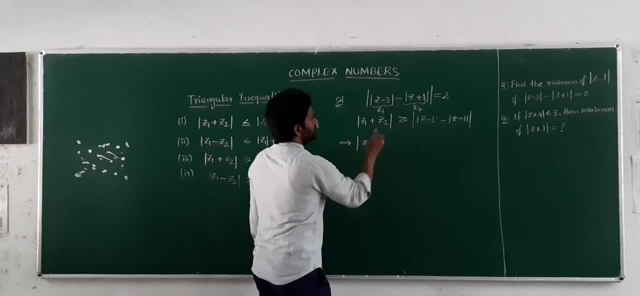 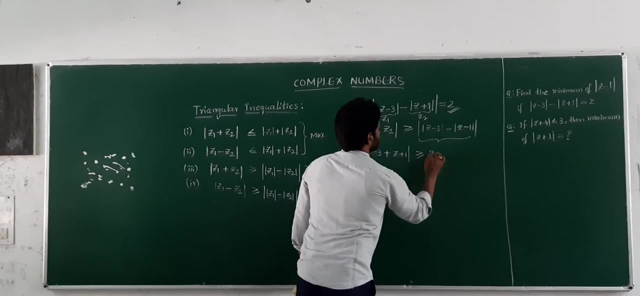 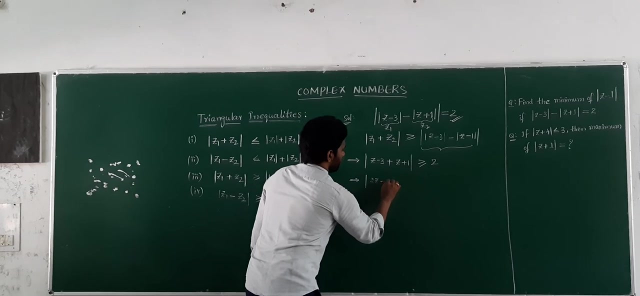 is: z1 equals to z minus 3.. z2 equals to z plus 1 mod of greater than or equals to, And this value is given as 2, which is greater than or equals to 2.. So if we solve this, and 2z minus 2, greater than. 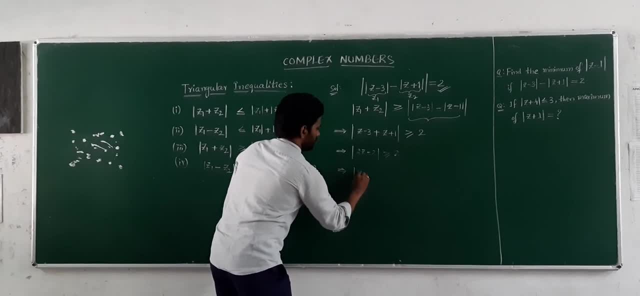 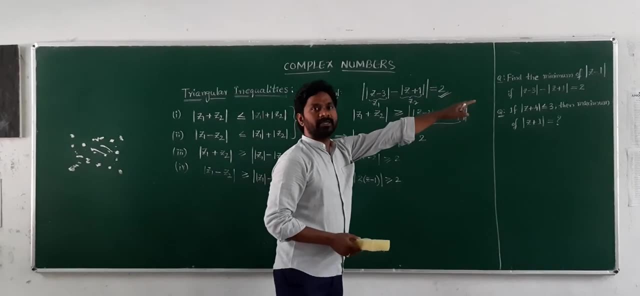 or equals to 2.. And if I take 2 as a common, I am getting the required condition. So that is z minus 1.. I need to get it as a z minus 1.. So I can write it as a z minus. 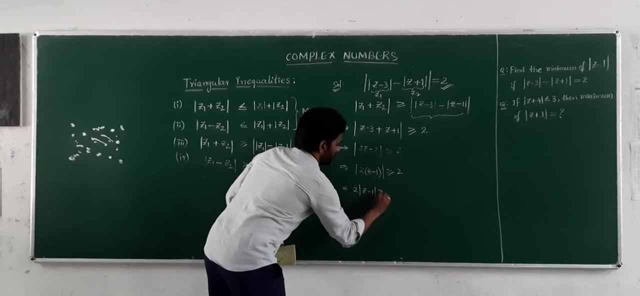 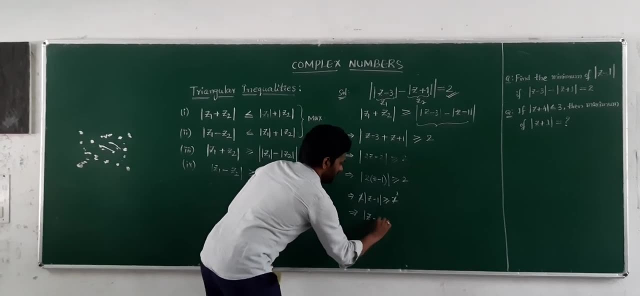 1.. So I can write it as 2 outside mod of z minus 1, greater than or equals to 2.. And if you cancel it out, this is 1.. Then I can say it is mod of z minus 1 is greater than. 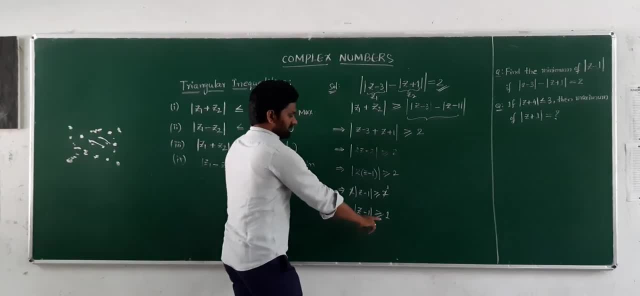 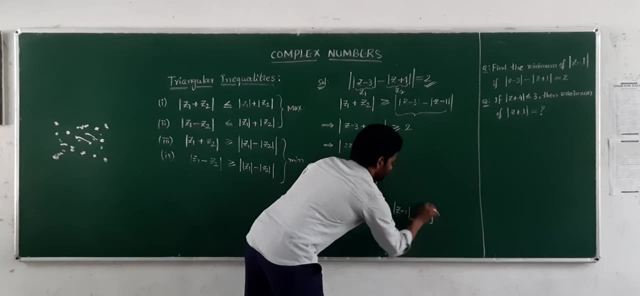 or equals to 1.. So that means the minimum. it starts with a 1.. Then the minimum value of mod of z minus 1 equals to 1.. Okay, the minimum value of mod of z minus 1 equals to. 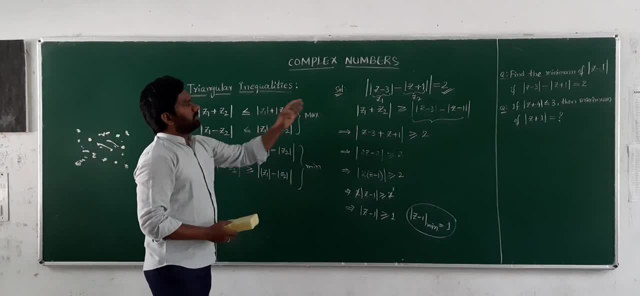 1. So by using the time-labeled equalities, we can find the minimum and maximum values of complex numbers.